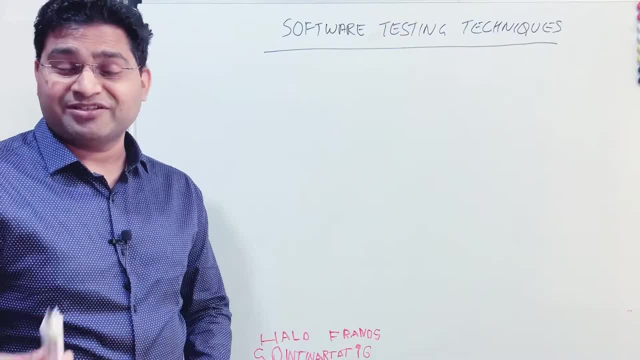 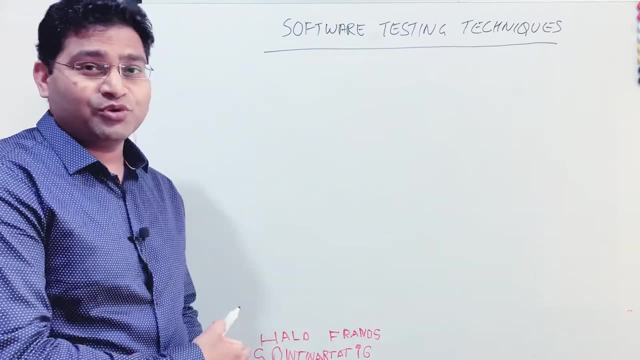 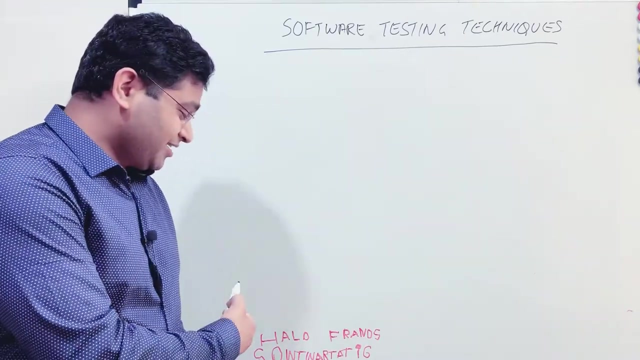 whiteboard and I can't delete it because this is written by my four-year-old son and he has requested to keep it on the board and not to erase it and record the video with this writing. So this is something related to what I already have been creating tutorial series on. He has 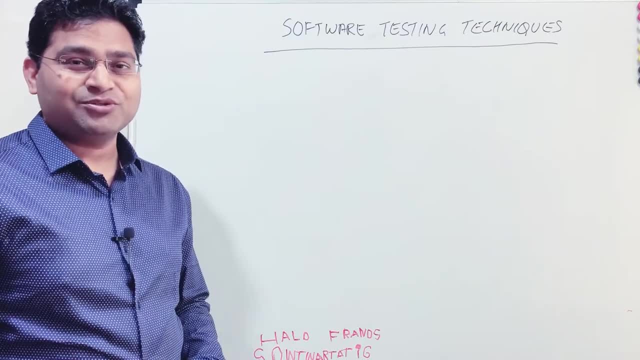 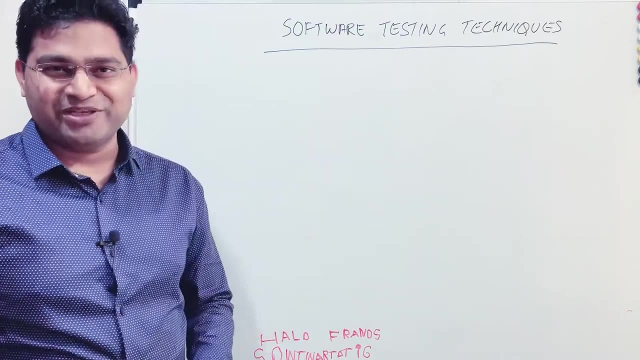 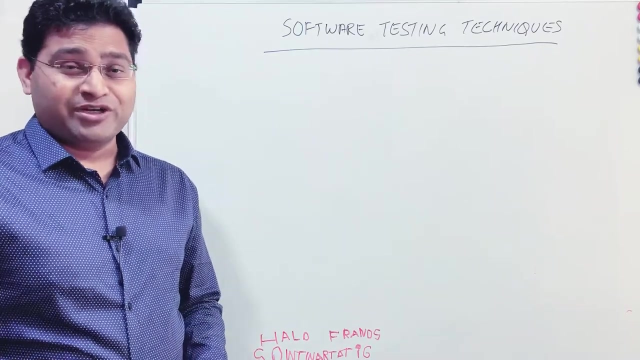 been listening to it and recently he has started writing. So he has started basically, or he has tried to write whatever I speak in the tutorial series or in the videos. So if you can guess what he has written Would be great. If you are able to guess, you know, comment in the comment section of this video. 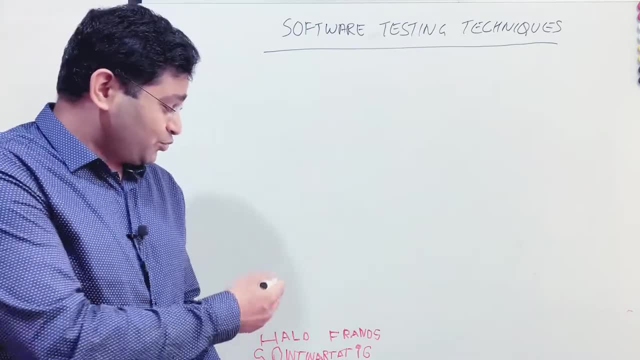 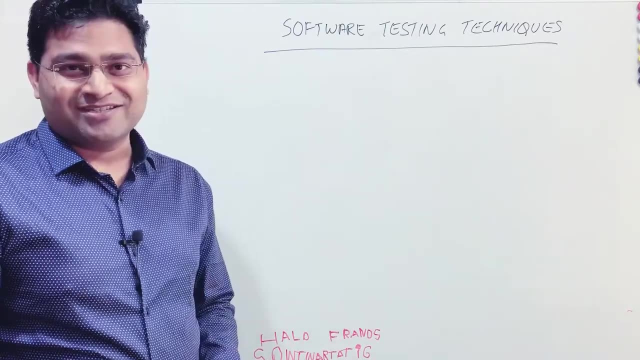 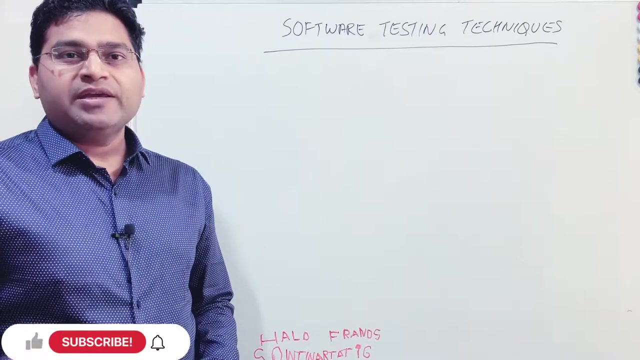 and he'll be really happy. So I'll record this video with this great piece of work on my board. And now let's get started with software testing techniques, or test design techniques. So, coming back to the actual topic, software test design techniques. Why is test design? 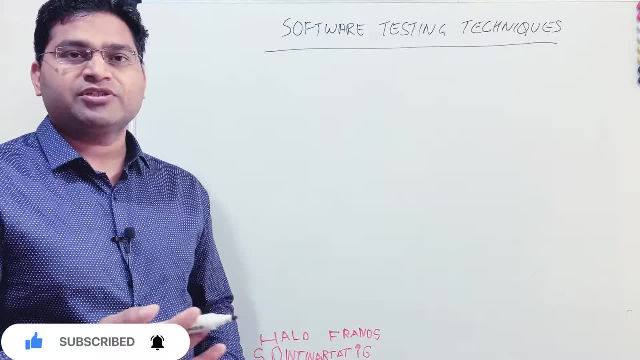 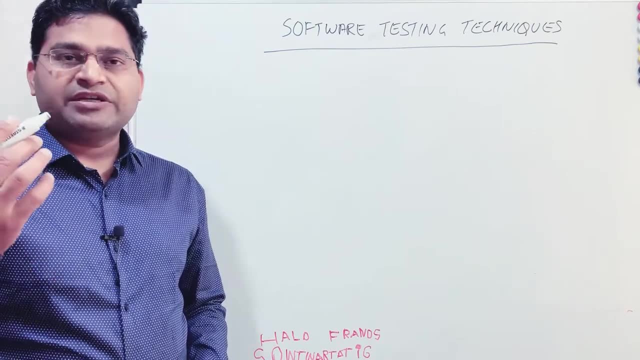 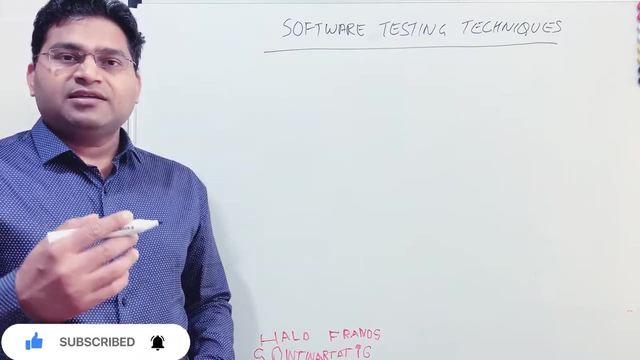 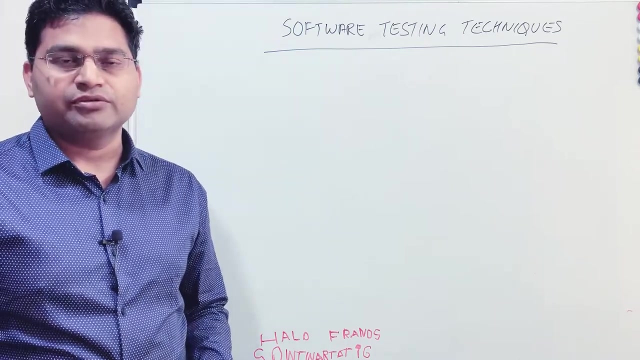 technique important. So if you have watched my previous tutorial on the principles of testing, we know that software testing principle, there is one principle which says exhaustive testing is not possible. So what that principle means is that even though it doesn't matter how hard you try to do exhaustive testing or try to cover all the scenarios that you want to, 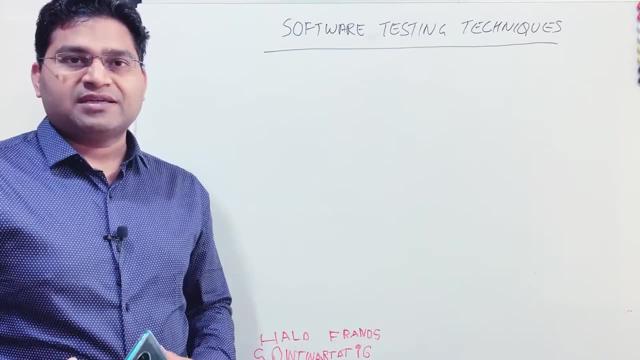 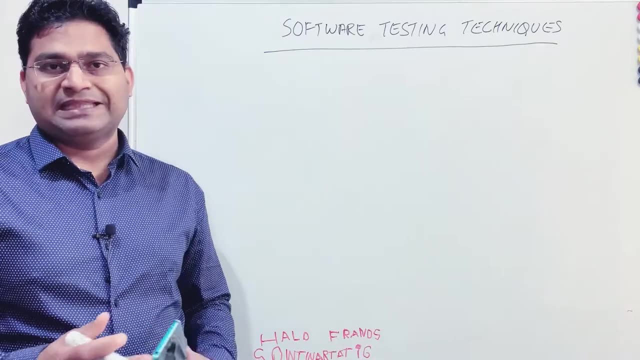 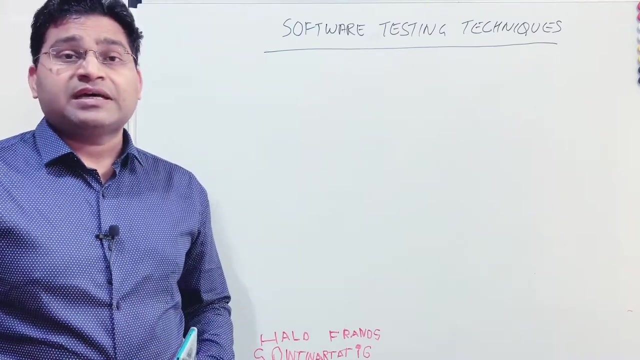 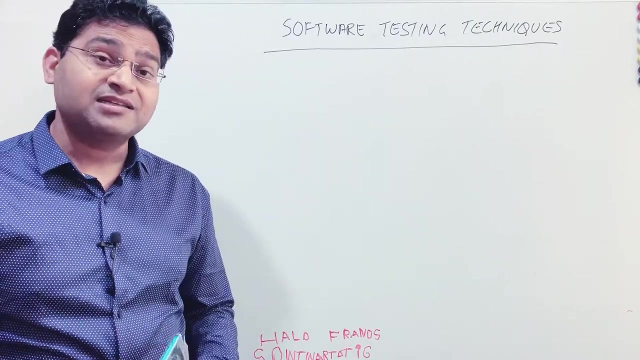 cover in your application as part of the testing process. it's still not possible to cover each and every scenario that is possible in the application. So because of that, we need to basically come up with the better ideas to design our test case, to write our test case, And that is where these software testing techniques, or software test design techniques, come in picture. Okay, so these techniques are: 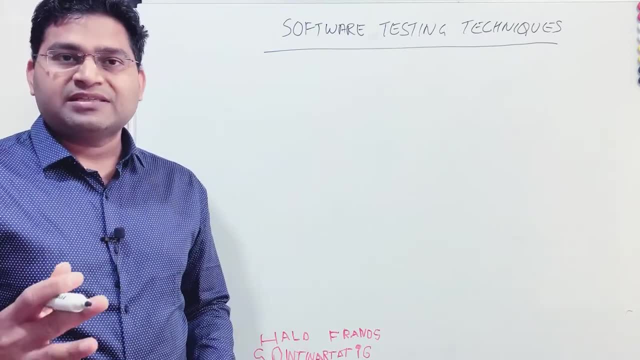 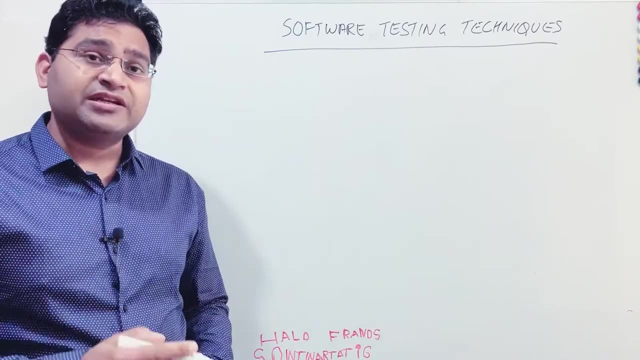 utilized or applied in writing your test cases Or you know. whenever you're documenting your test cases or scenarios, you apply these techniques or tags. you jump on the test test techniques and come up with the scenarios so that whichever test case you write, 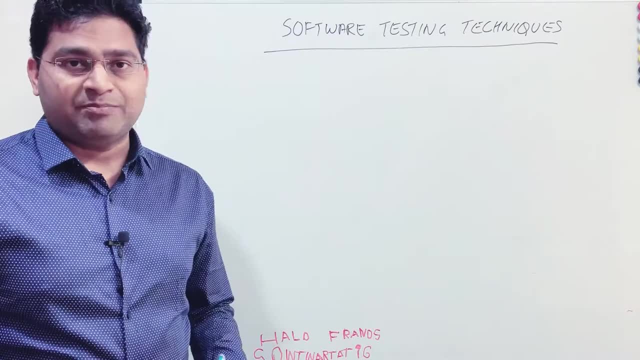 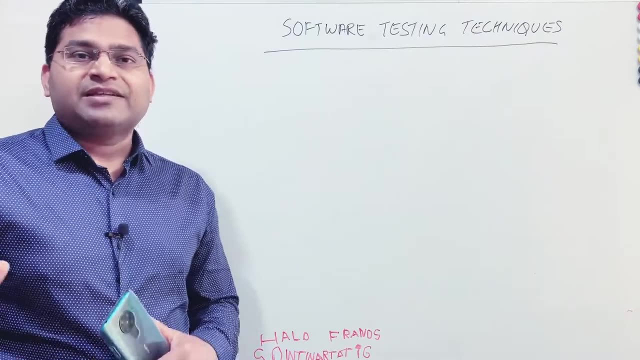 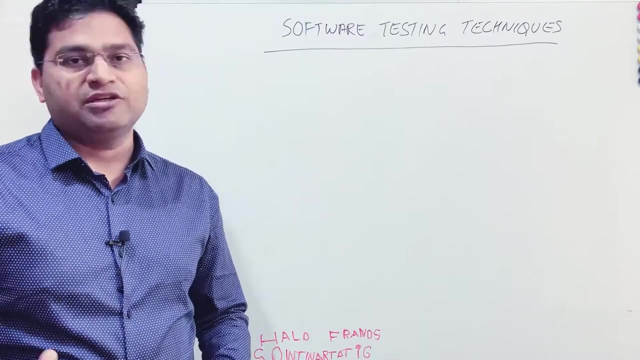 those test case provide you the maximum coverage of the application. So your testing is not random. You are not just randomly testing here and there. You apply the techniques and then you write the test case so that you get the maximum benefit of the testing that you are doing in your 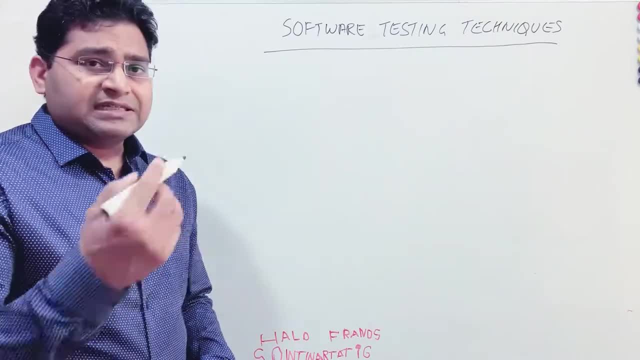 application. All right Now, if I talk about the software testing techniques, I'll cover all you know. black box t s design tips, I'll cover allu. So you know in fact all the test test: Civilę t a. 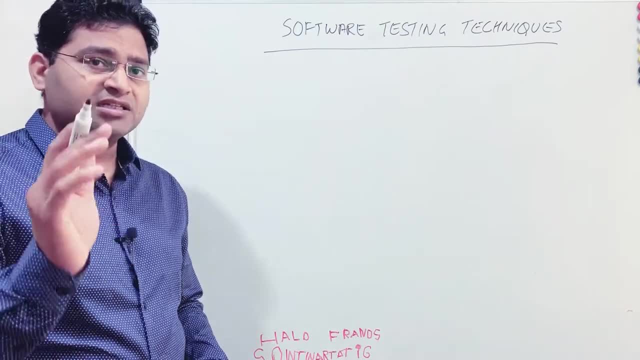 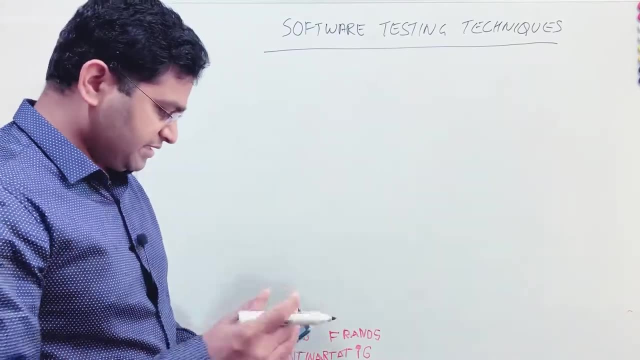 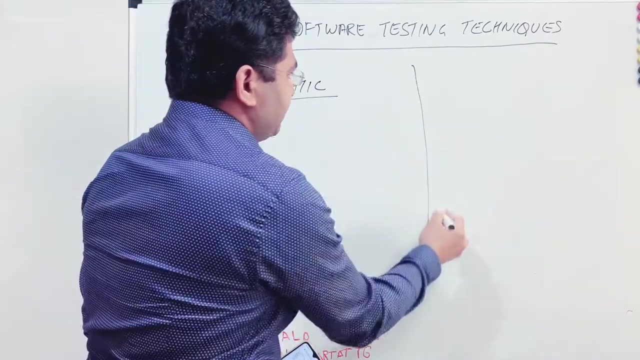 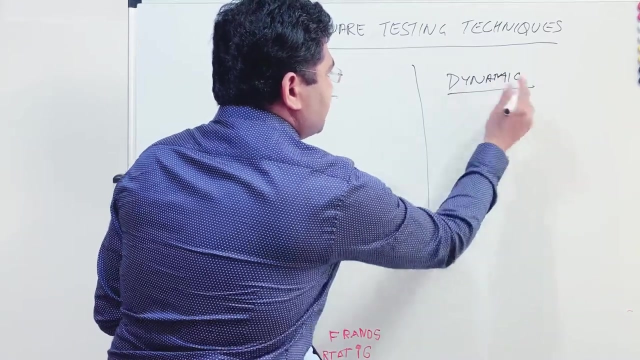 test design techniques in detail in upcoming tutorials, but in terms of high level, what all software testing techniques are possible. so we can see that software testing can be categorized into static and dynamic. right, so i can say static and dynamic. so so these are two broader categories of the software testing. so in the static testing we have understood about the execution or 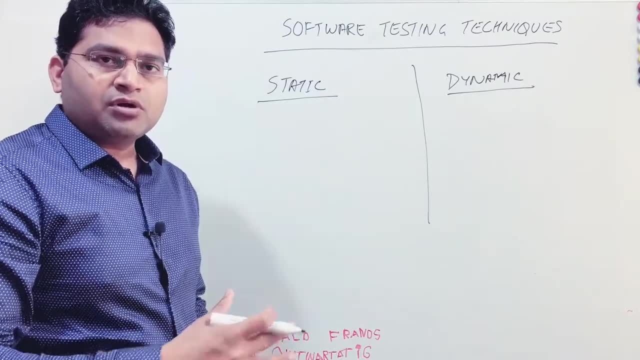 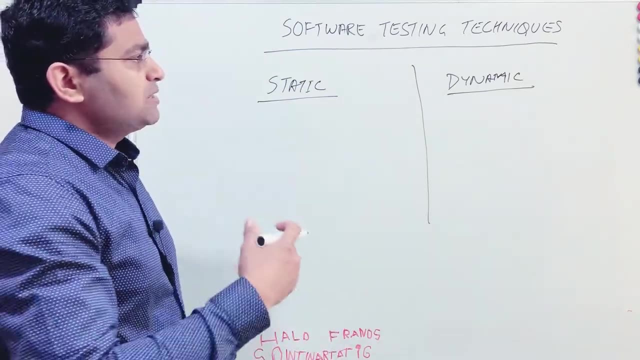 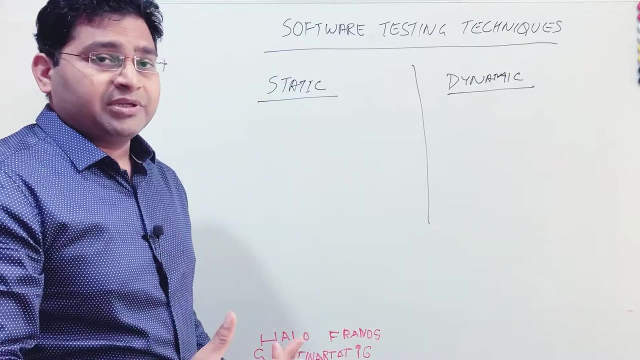 basically the testing of the software or the document or anything related to the application without executing the code. so that is static testing. when we say dynamic testing, it is when you execute the code and you actually launch the application and you test the application. so that is dynamic testing. now, software testing techniques are applicable in both cases. so in 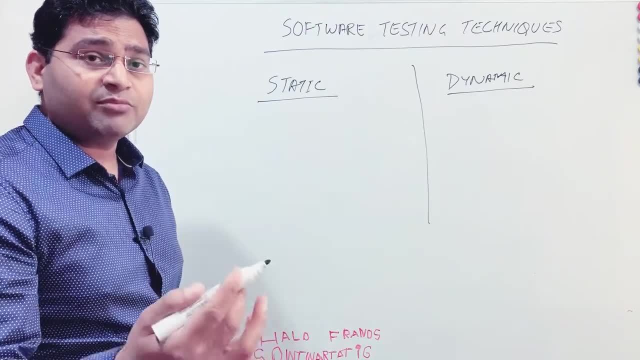 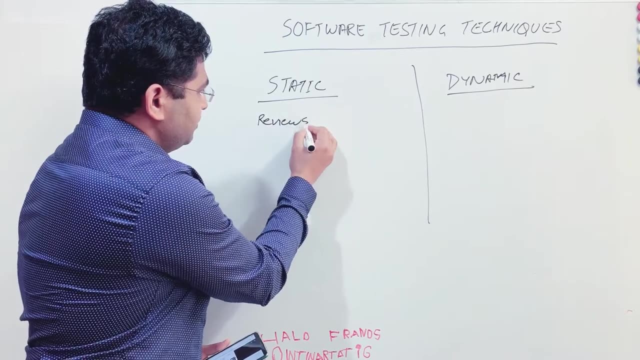 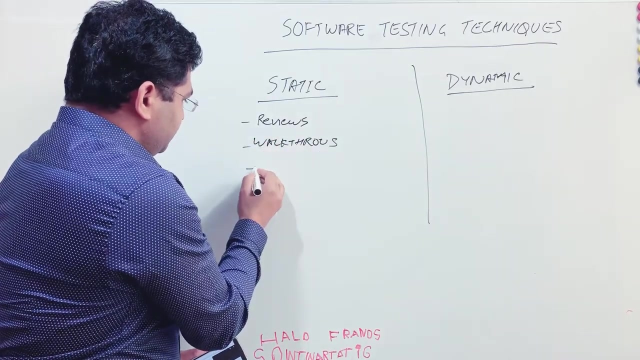 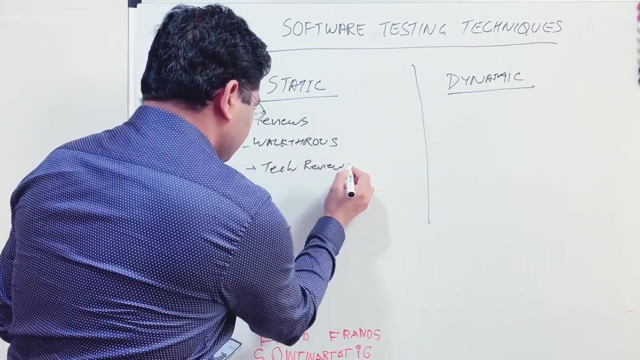 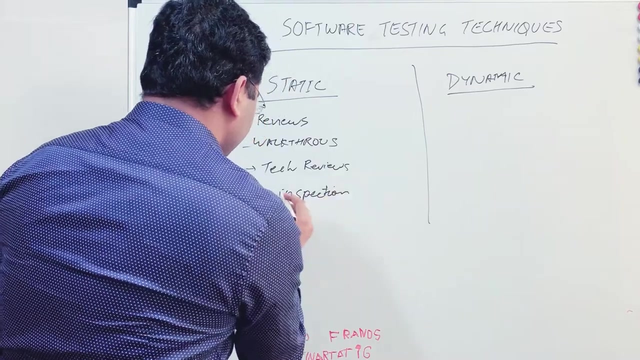 in static testing, testing techniques or in static testing, some of the techniques that you utilize are, you know, say, for example, reviews- walkthroughs- okay are. the other one is technical reviews, tech reviews- okay, then you have inspection right. so these are, you know, some of the static testing techniques. 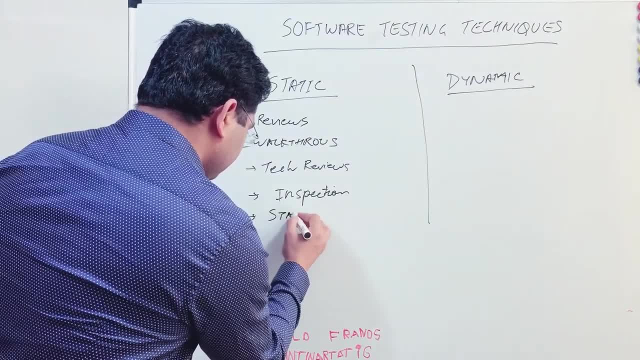 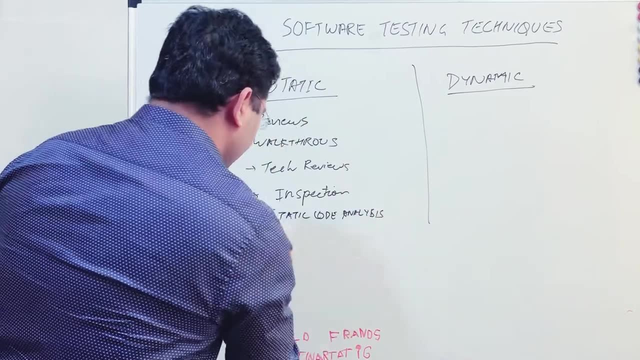 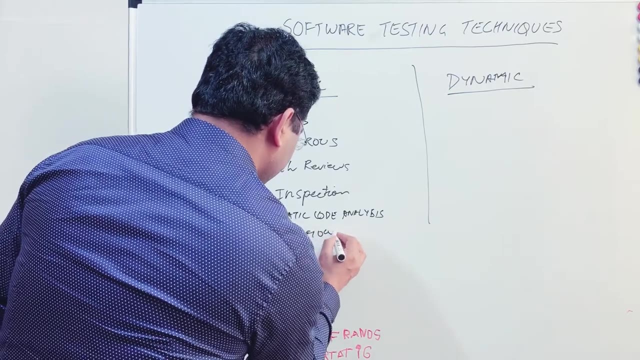 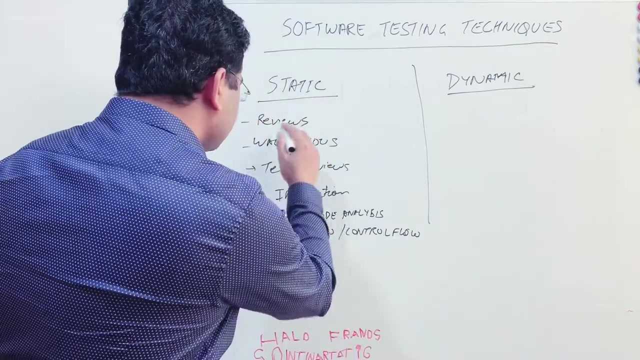 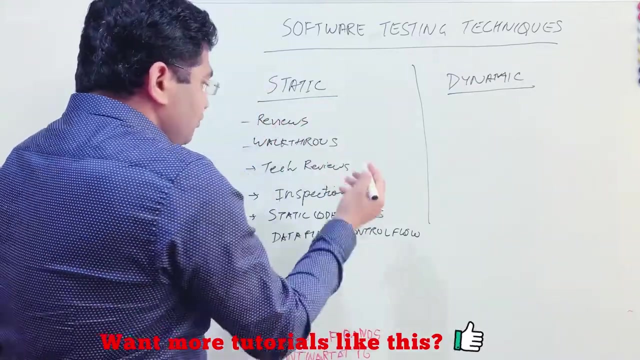 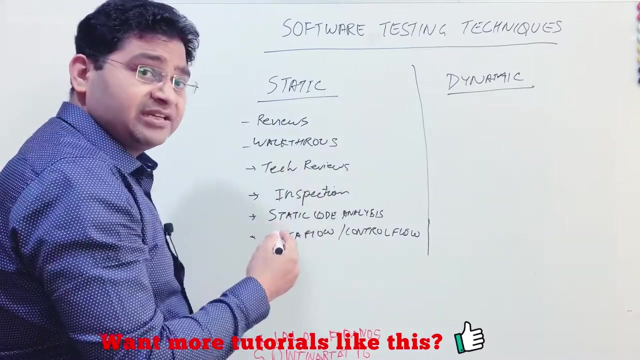 um, then you have, you know, static code analysis, all right. and you have, you know, data flow. you check the data flow, you check control flow, okay, so these are some of the static testing techniques that you can, you know, apply in the static testing. now, if you go through my istqb, you know tutorials- you will see all these static testing techniques. 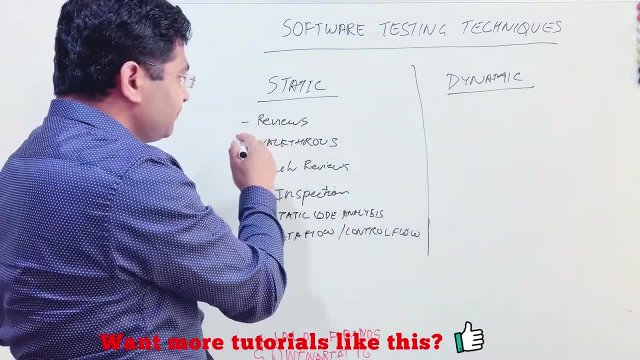 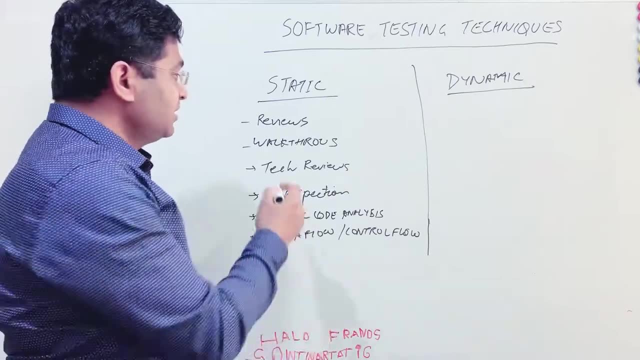 covered in detail so you can you know. go through those tutorials and you will be able to understand if you are preparing for istqb certification as well as part of the series. then you can go through those videos and understand what exactly reviews is. what is tech reviews? what is inspection? 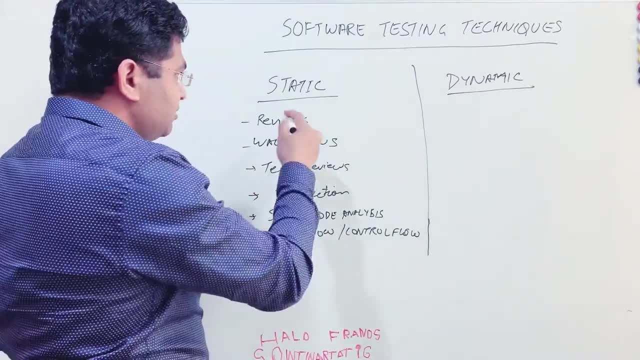 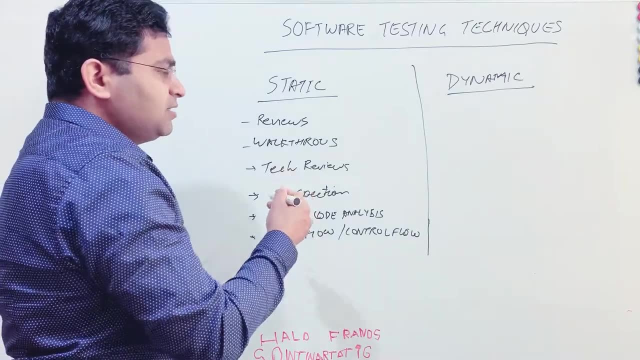 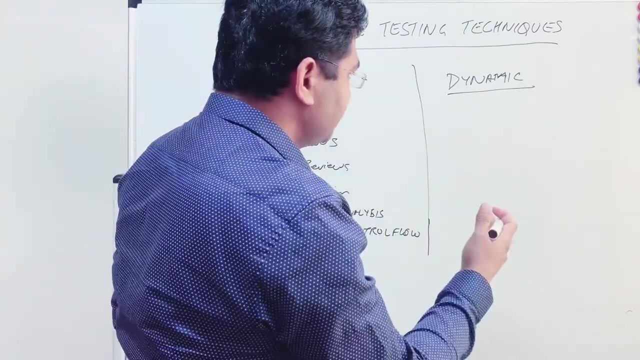 how formal they are, how informal they are. all that is, you know, uh, explained there. so these are some of the static testing techniques that are applied to basically do the static testing for the, any application or for any software. now, when we come to dynamic testing- now dynamic testing- we have you. 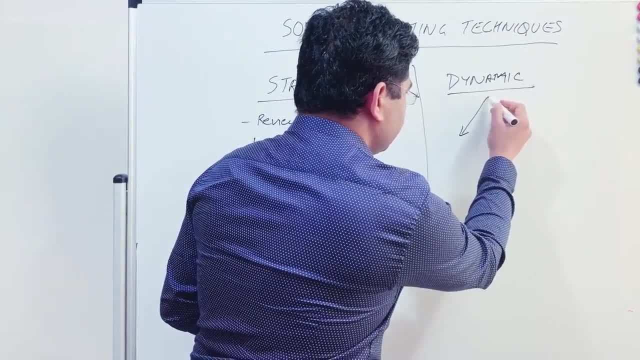 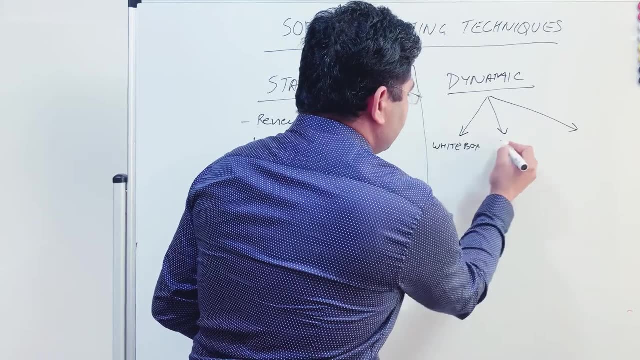 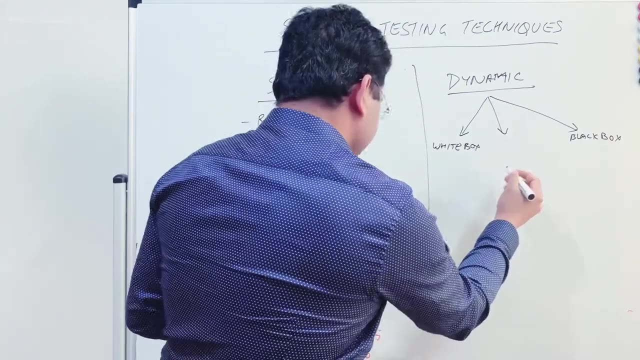 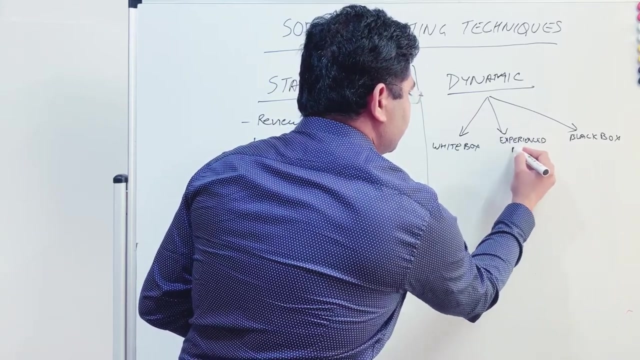 know two. um, basically, we can say we can categorize dynamic testing at the high level as white box- okay, so white box, black box. and then we had this experience based- okay, so experienced based- in which we have this exploratory testing- right, so, we have exploratory. 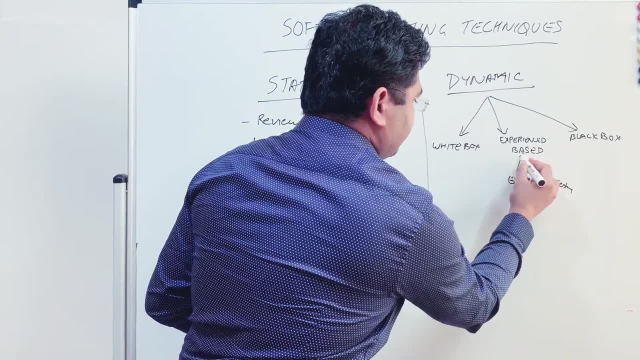 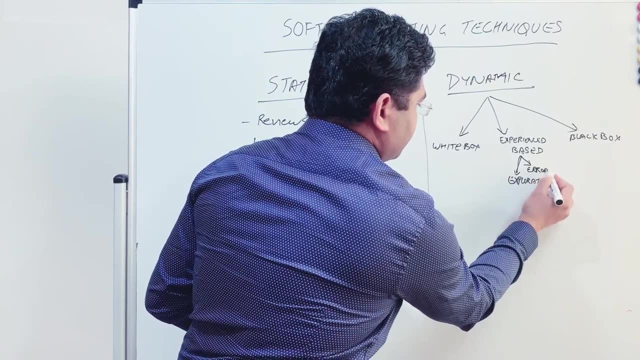 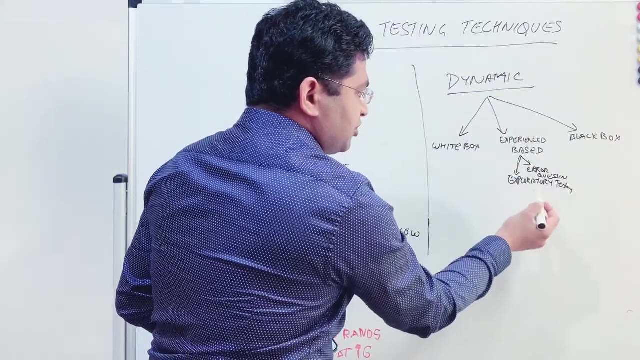 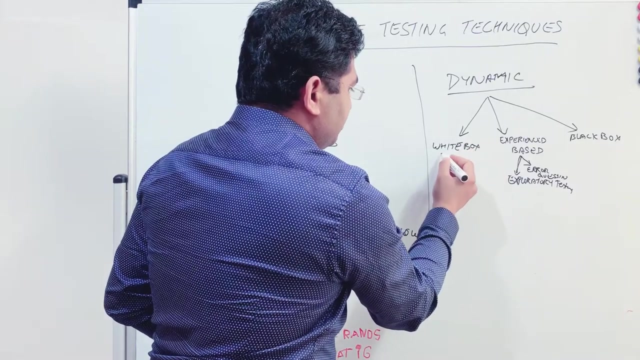 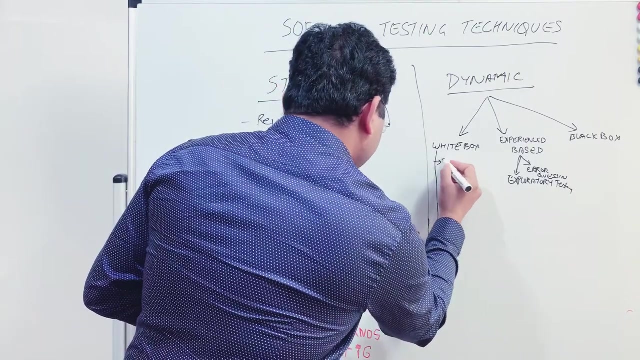 testing. and then we have another one is error guessing. okay, so in the experience based, you apply exploratory testing or error guessing techniques in the dynamic testing approach. now in the white box you have several white box testing techniques, so some of the white box testing techniques are. so, for example, you have statement coverage, which is 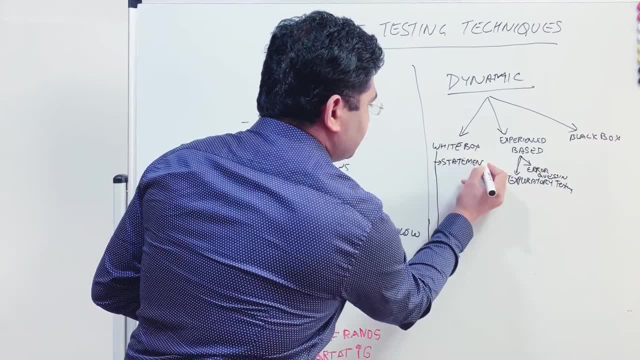 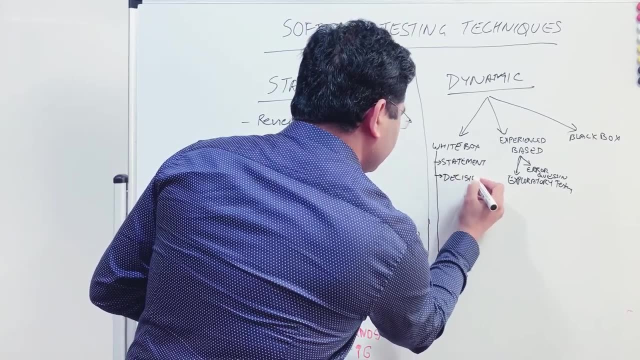 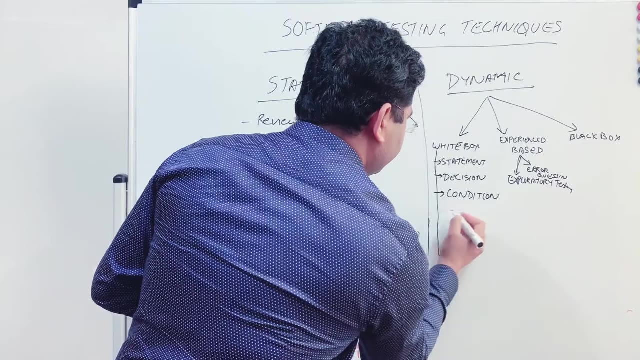 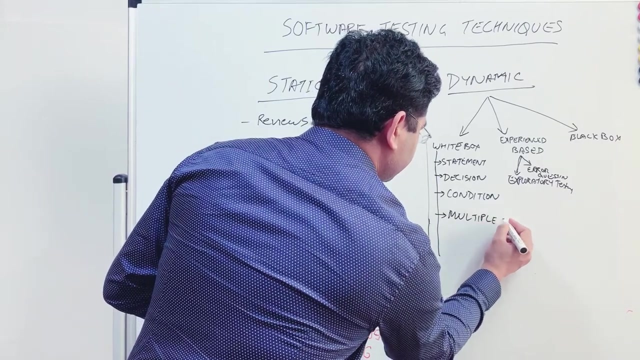 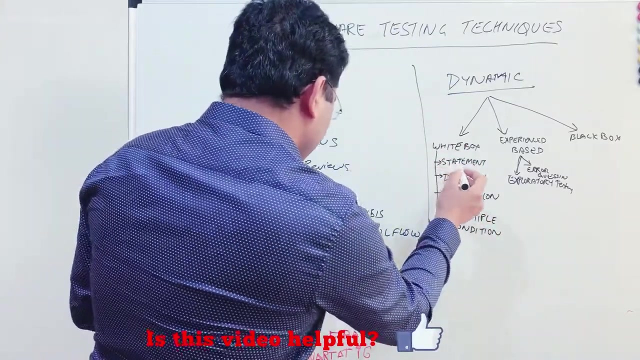 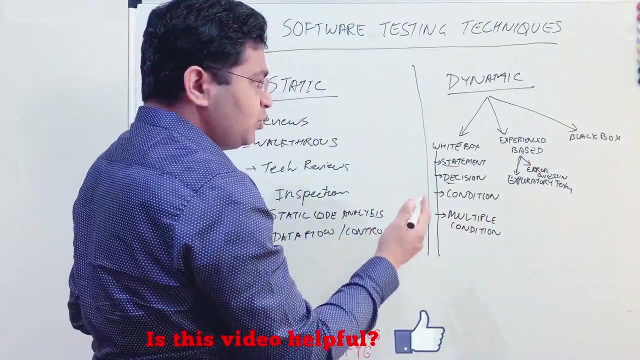 very important. so statement coverage, then you have decision coverage, then you have condition condition coverage, then you have multiple condition coverage. okay, so multiple condition, right. so in the white box testing technique you applied some of these techniques- statement, decision, condition, multiple condition- and verify whether the code that has. 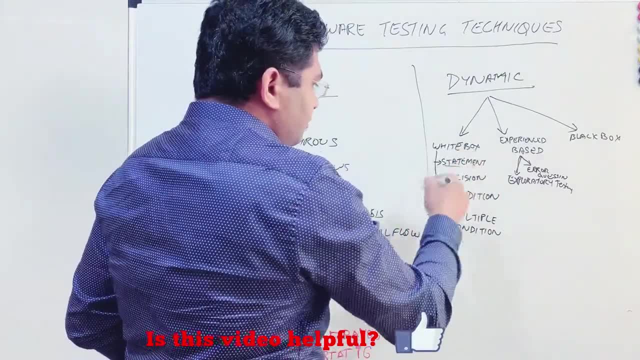 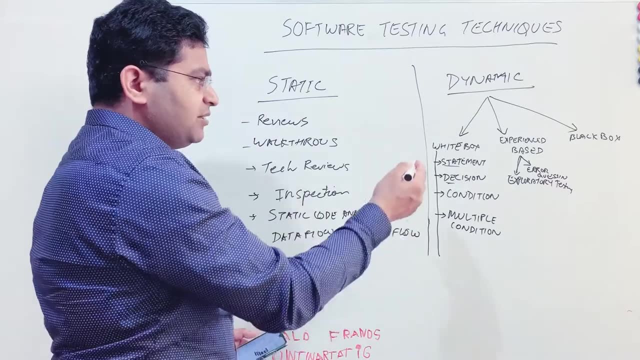 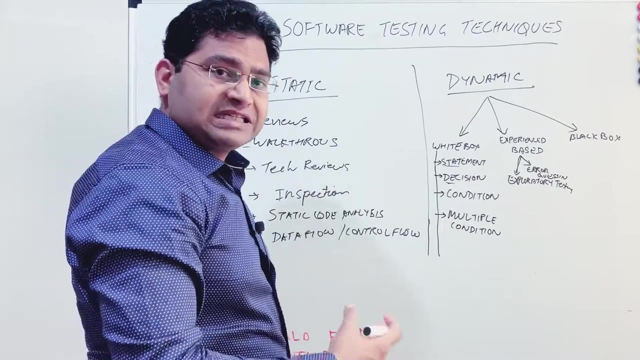 been written as part of the application covers all these. you know white box testing technique, so you apply these techniques and ensure that everything is working as expected and with these techniques, when you apply, you ensure that you are getting good coverage as part of the testing. okay, now in the 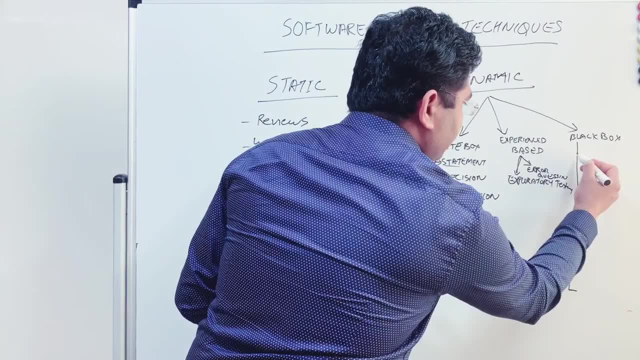 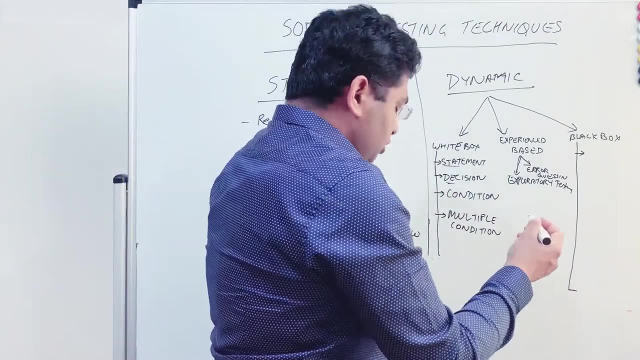 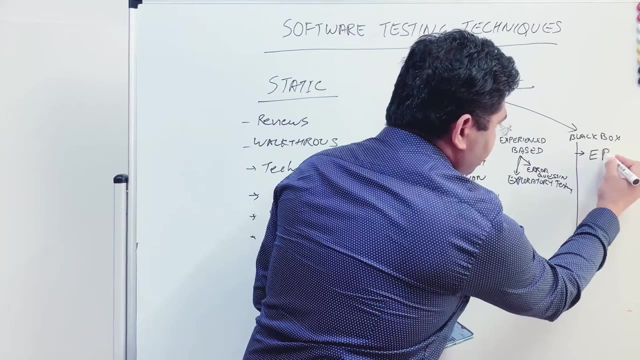 black box technique. these techniques, the black box techniques, are very, very important and we'll be covering these in a lot more detail. so when we cover the black box tech, testing techniques, which is basically, you know, equivalence partitioning right, so we can say EP, boundary value analysis, you would have 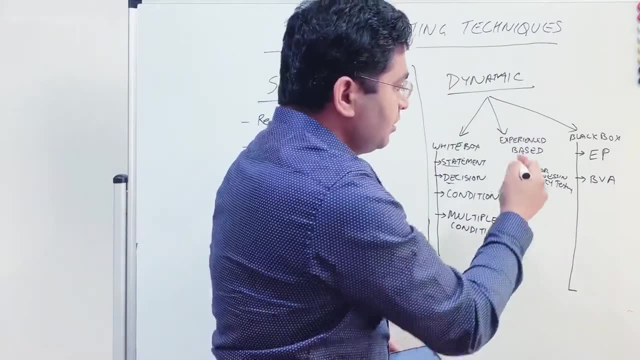 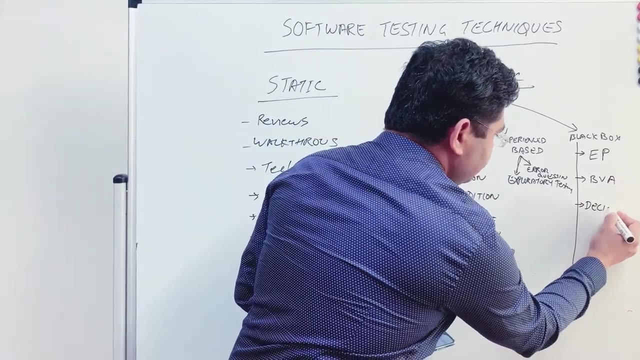 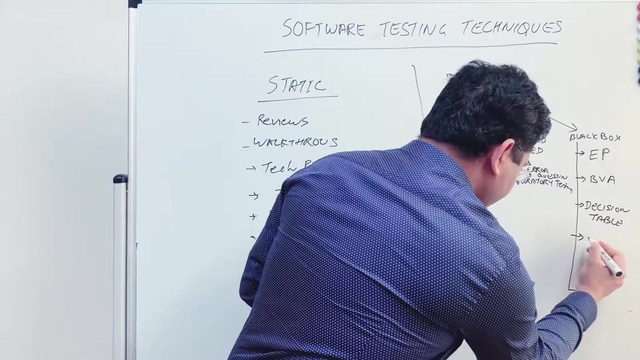 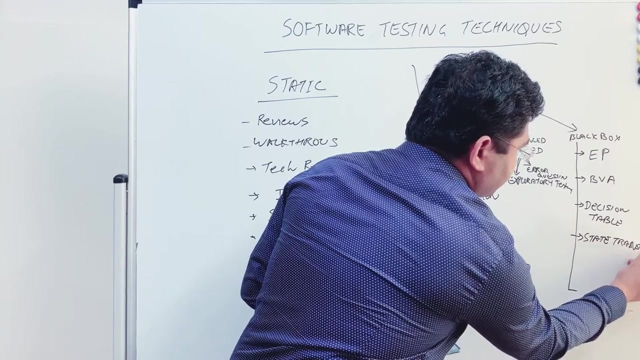 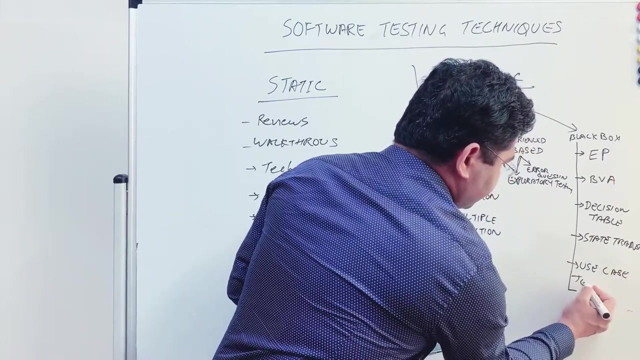 heard about these words will explain with example all these concepts. so, equivalence partitioning- boundary value analysis, then a decision- partitioning- boundary value analysis, then decision table, decision table. then we have state transition, state transition and we have use case, use case testing. okay, so these are some of the black box testing. 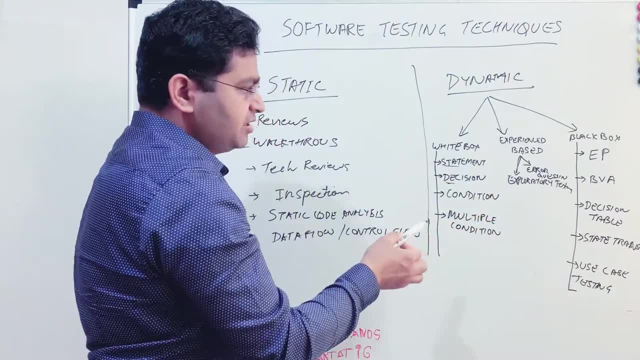 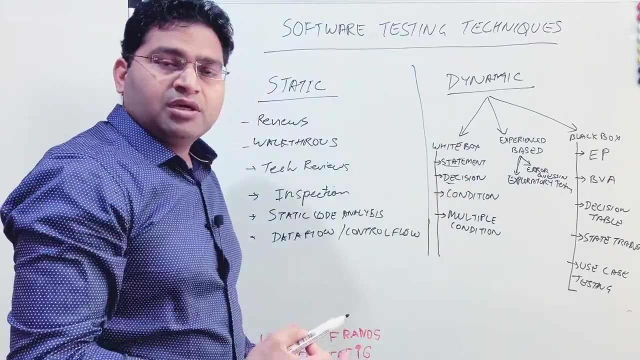 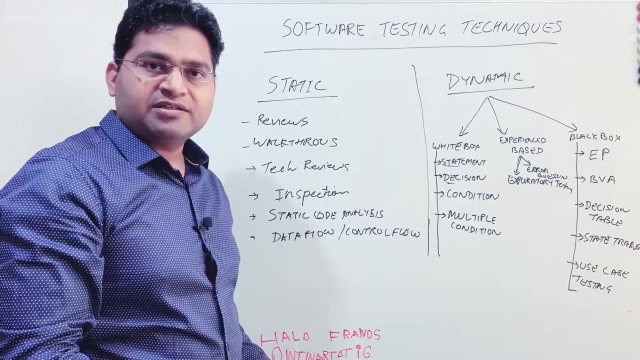 techniques. so equivalence, partitioning, boundary value analysis, decision table testing, state transition, use case testing. these are very, very important because, if you are doing manual testing, these are the techniques that you will be using day in, day out and, knowingly and unknowingly, most of the testers or members of the team do apply these. 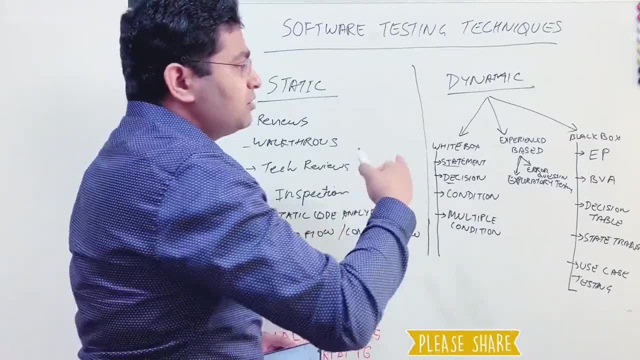 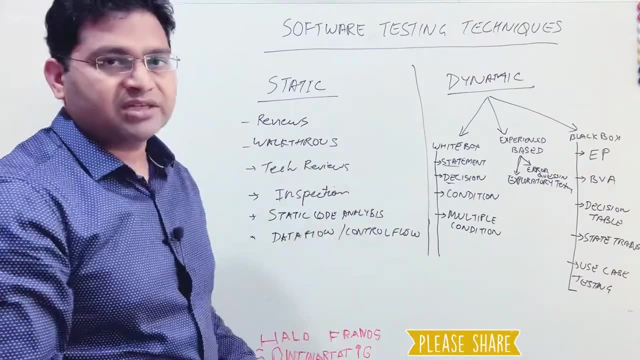 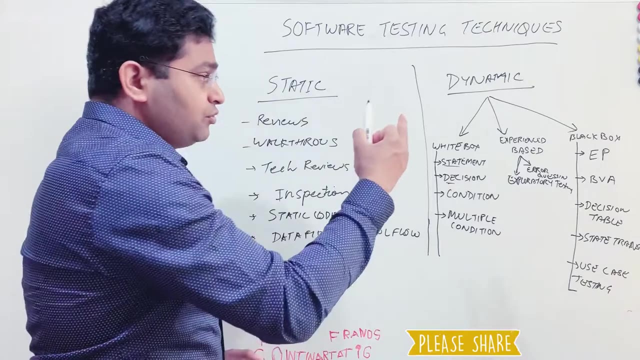 techniques, but most probably you might not be aware, but you are still. somehow. when you are documenting a test case, you will be covering some of the equivalence partition or you know boundary value conditions you will be covering or the values will be covering as part of testing. but if you know these concepts, 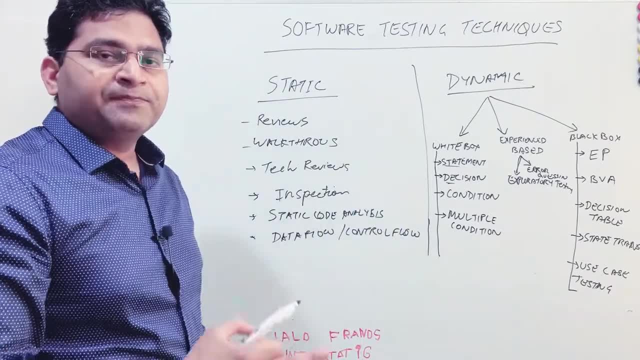 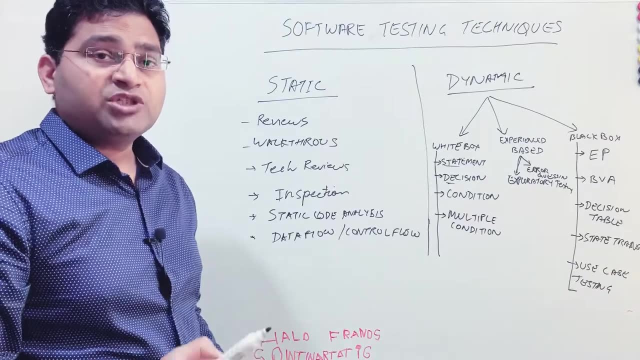 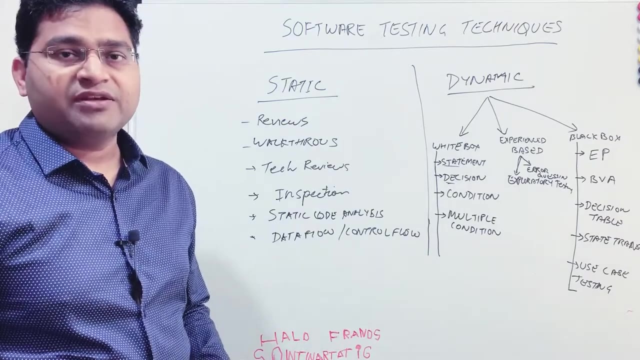 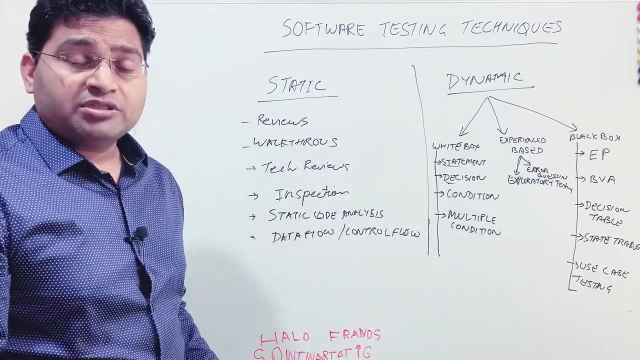 you will definitely be able to apply these and apply all these techniques properly when you are designing your test cases, which will help you a lot in getting a wider coverage and better coverage in terms of testing for your application. okay, so if we talk about static and dynamic testing as part of the ISTQB tutorial series, which is already on my 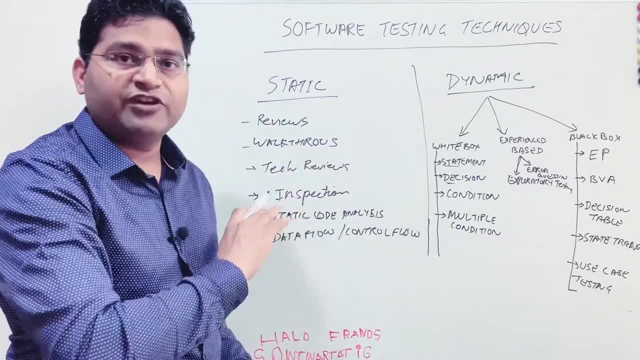 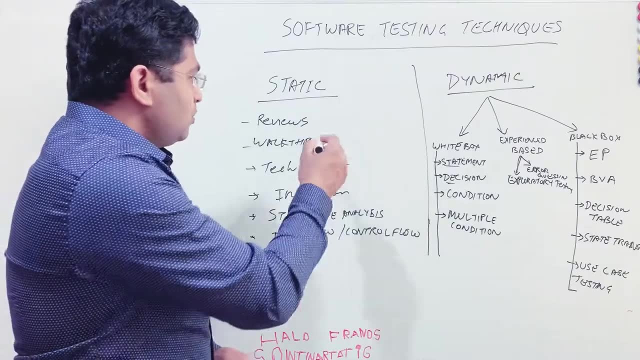 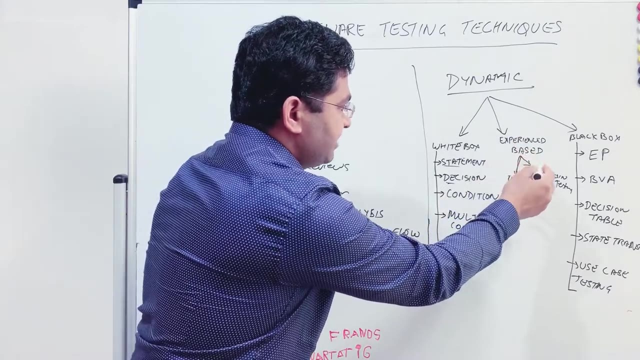 youtube channel. all of these things are explained very much in detail and cover all the aspects of the ISTQB certification. now I won't be covering all these static testing techniques, dynamic testing techniques and you know this error guessing as part of this series- software testing tutorial series, because this